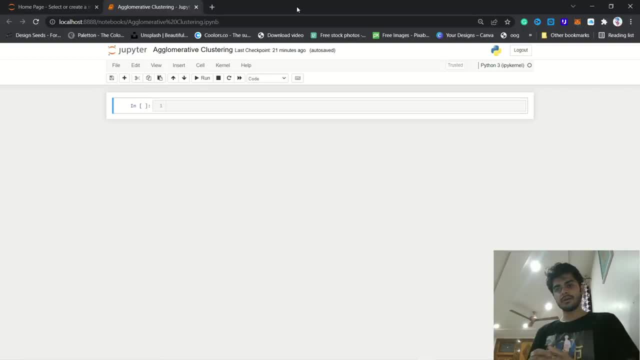 We do filtering and we can explore our data. We can perform operations, We can perform our data with pandas. And what is matplotlib? Matplotlib is actually a library which helps us to plot a graph out of our dataset, to visualize our data. 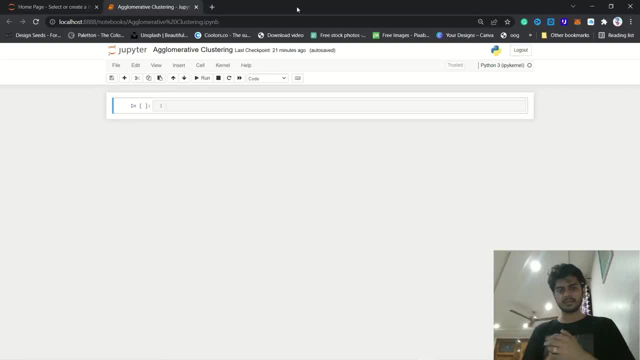 So these three libraries we will use in like in starting our agglomerative code And let's import these three libraries and we will continue from there. So I will say: import numpy As np. Why am I writing as np? 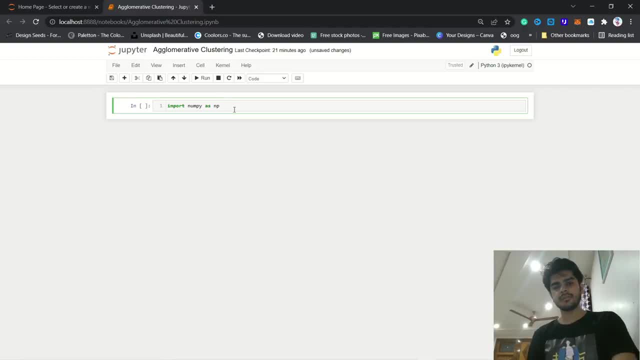 So I want numpy to be represented as np, because writing numpy every time is very tedious, Like if I have to work with some data and I have to write numpy every time, that will be very tedious. So I am saying that numpy is as np. 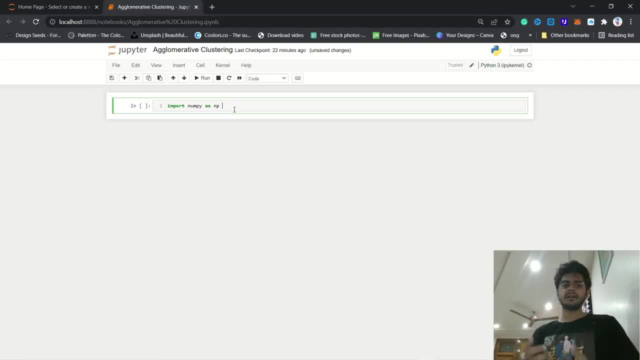 Whenever I will say np, you should understand that I am talking about numpy. Like then we will go and import numpy. So import pandas as pd And import matplotlib as pld. So these are the three basic libraries which we will going to use. 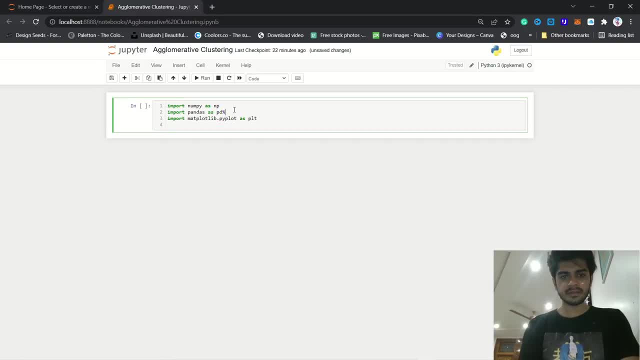 And we can do one more thing that we can say: percentile, Yeah, Percentile Yeah, Matplotlib inline- What matplotlib inline does like when we plot our data. if we don't write this thing, it will open a new tab for visualization. 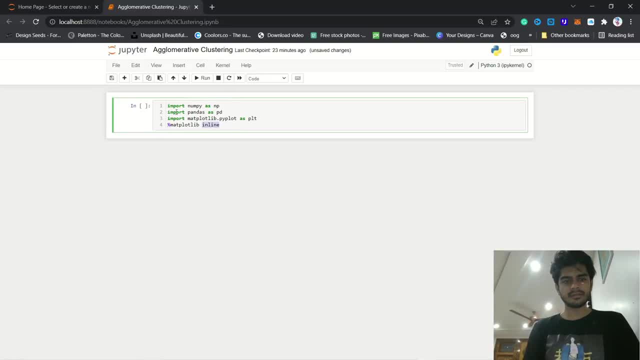 But if you include this, it will give you that data visualization here, only in this, in this uh, where we are working. so this is uh why we are uh like saying that, uh, percentage mat plot in line. i want data in this window. so let's run our code and let's see. it will take a. 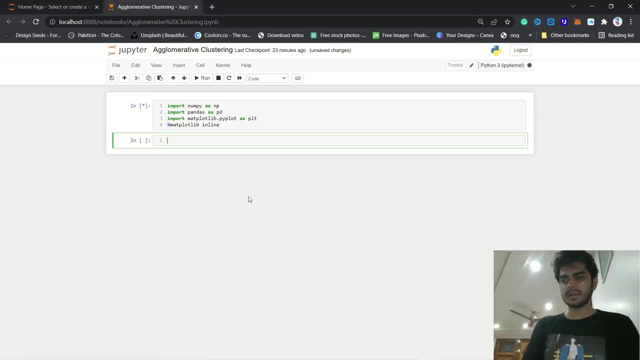 few seconds or minute to import libraries and then we will go and import um, our data set, which is zoocsv, and we will see whether, what, what are we working with in our data set and how we can get an information of about our data set um by pandas. we will do that, okay now. uh, we imported our 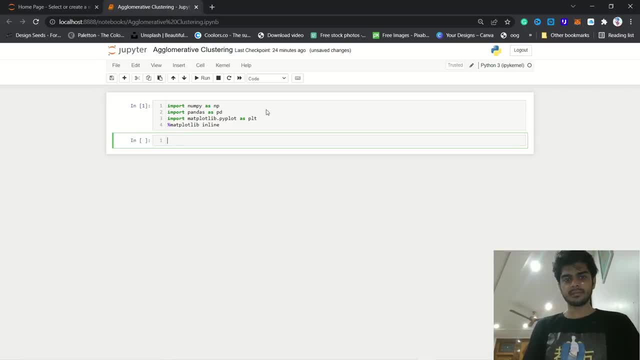 library successfully because we have. we don't have. our idea is not showing any error, so let's import our data. let's say: this is: i'm making a variable which is known as data pd for uh. pandas dot csv. like uh. why we are using csv, read csv. sorry, why we are using csv. csv is. 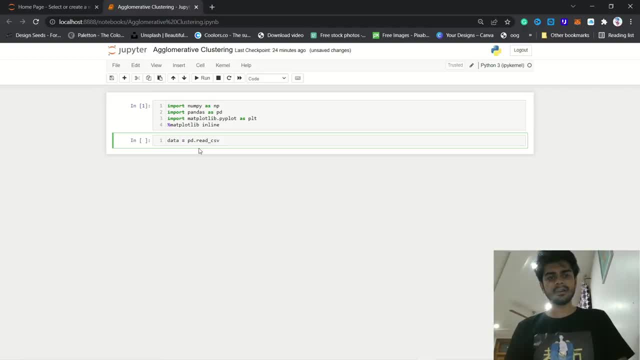 basically comma separated files. it is used for comma separated file and we are using that pandas dot read csv. that read this csv file which i'm going to import and that is zoo dot csv. so it will uh like, uh, take the csv file and read it and let's say we want an information from our csv file. 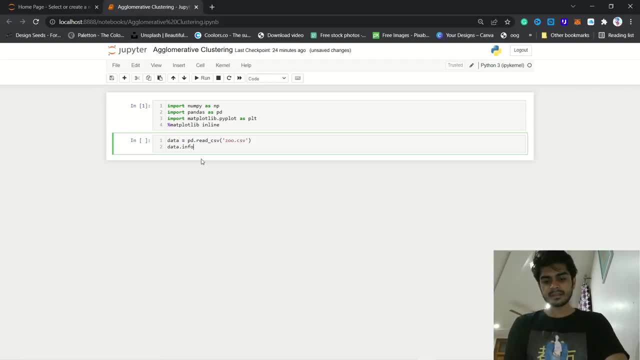 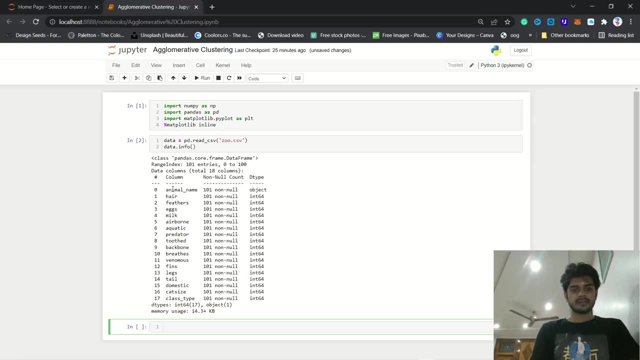 so we will say data dot info and this will give us information about our file which we are working. so, as you can see, we have columns uh animal name here: feather egg, milk, airborne, aquatic predator, backbone animal, sphinx, breaths, legs, tails and like uh. all kind of uh data is there and int64. 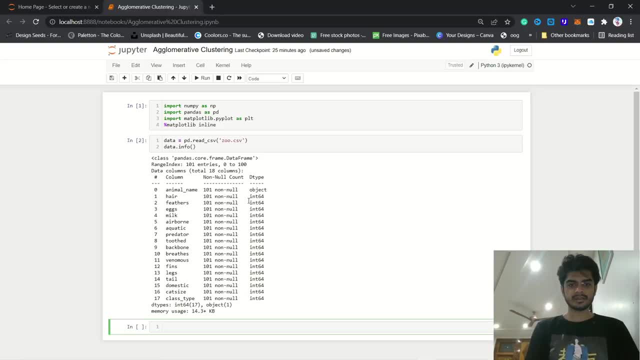 represent that this is an integer value. see, all of this is like integer value and this is an object and my name is an object and uh, yeah, this is the data which we are working with. so, and there is total 101 entities which have 18 columns. we have over 18 columns in our data set, including 0: 0 to 17 is actually 18 columns. 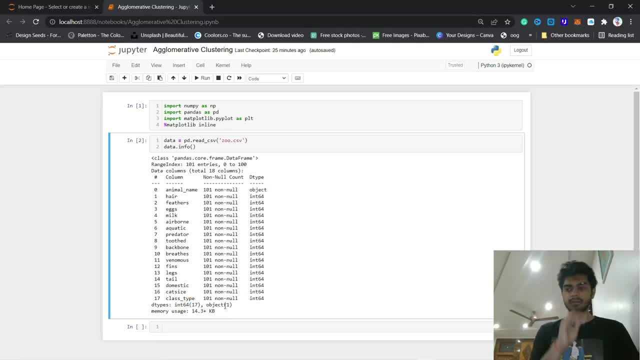 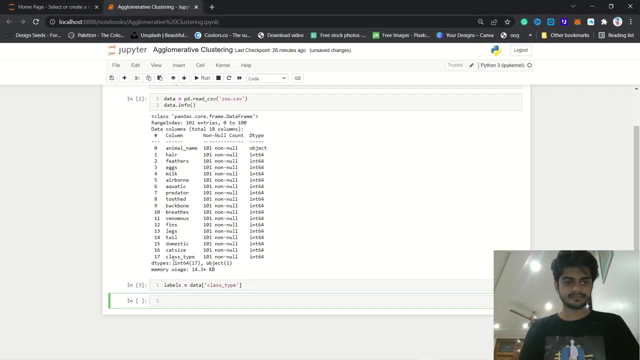 17: uh in 64 data types and one object data type. so we got this: um, uh like uh information about our data type. let's go and make a variable label and say data and uh, last time. basically, we uh say data is destined to storing data and that information does not. uh. 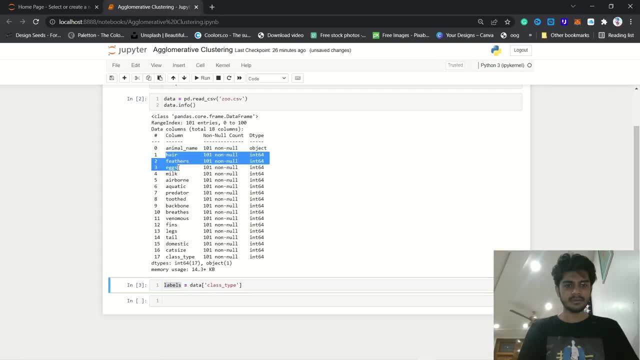 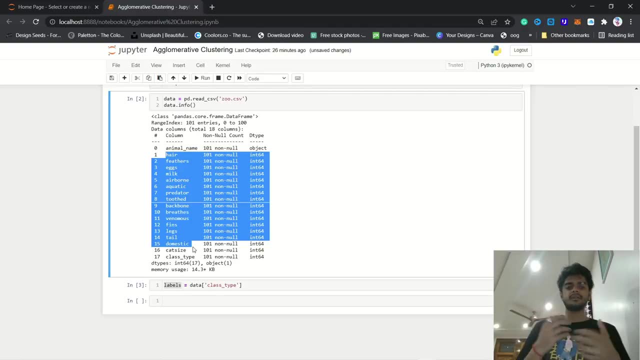 exhibit that, because what we're had is busy data and so you can just know, like this direct dependence on our data set. I'm using dependent and independent variable, which is not true with the supervised learning, but in a sense which I'm saying that let's take. 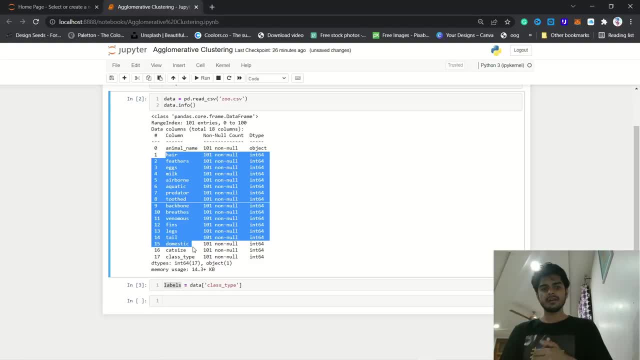 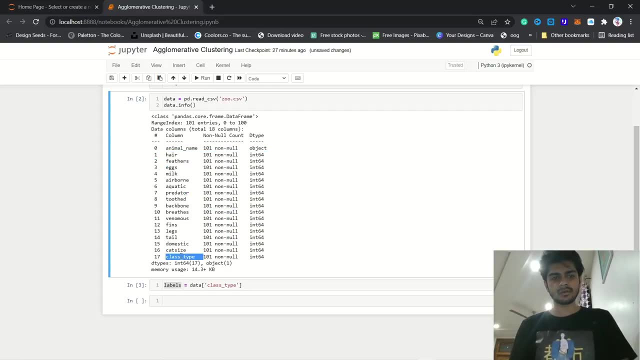 something out of our data set which we can use to predict our data set. So I'm using like class type column for that. So now let's see how many unique values are there like in our data set? Again, like numpy, library dot, uniqub and p dot. unique labels: Label. 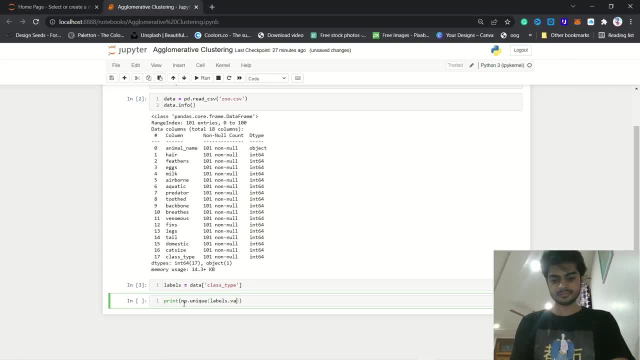 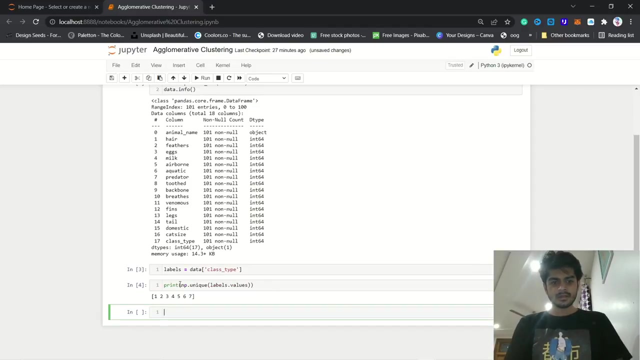 dot values. So this should give us like unique values which are present in, like our label, which is class type, which is this Unique value in this? So I think it will be label underscore. So it is giving us 1,, 2,, 3,, 4,, 5,, 6,, 7,, 8,, 9,, 10,, 11,, 12,, 13,, 14,, 15,, 16,. 17,, 18,, 19,, 20,, 21,, 22,, 23,, 24,, 25,, 26,, 27,, 28,, 29,, 30,, 31,, 32,, 33,, 34,, 35,, 36,, 37,, 38,, 38,. 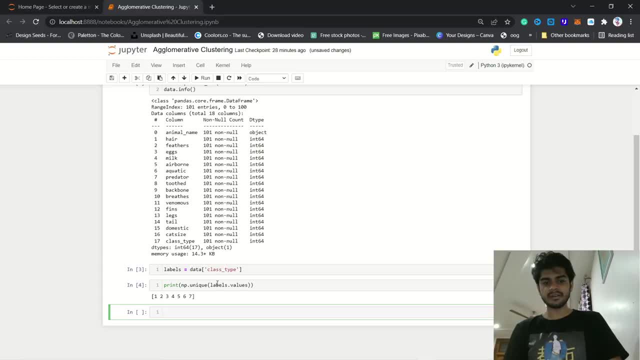 39, 40.. So these are like unique values which are in our this class type. And, yeah, it is like data array of a number: 1, 2, 3,, 4,, 5, 6, 7.. Let's go ahead and plot a graph And 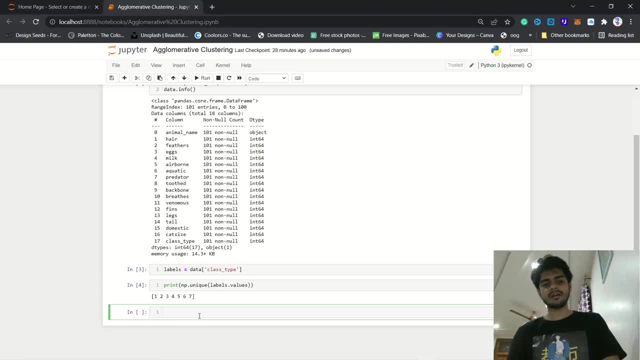 if you are thinking, what I'm looking into in this is that is like taking help of my note which I like made in So that I give you correct information And you get correct information. So let's say figure, If you want to like. these are variable name which I am writing Like you can have. 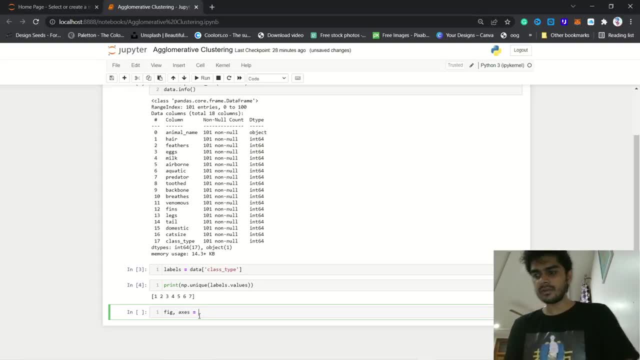 your own variable name, whatever you want. So figures xs, plt or matplotlib, dot, subplots, And theoretically what it should do. It should create a variable name, It should create a subplot. And what kind of subplot. Let's say We are going with labels. Labels, I guess. 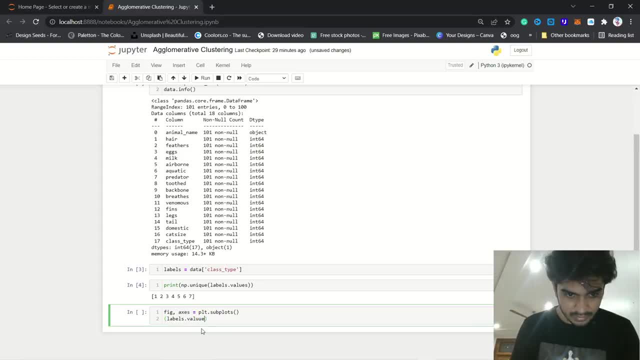 Labels dot value. Value is values Value count. It will give us the count of our value Label. How many values, How many, How many? How many values are there in label? Then it will plot that thing to ax, Which is axis. 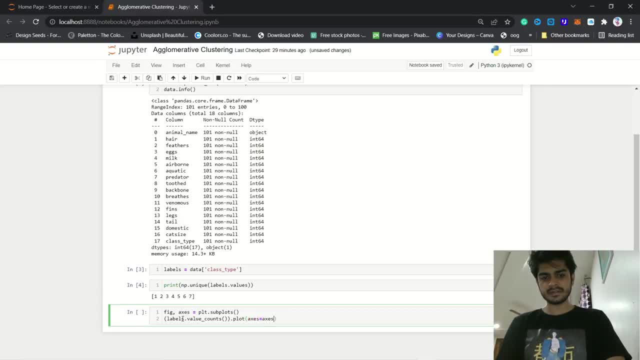 Or let we have make label of this And we want the graph type to be bar chart. So let's go ahead and say bar And this should give us a like bar graph And what we can do is that we can say that features See in like supervised learning. we have labels, But in 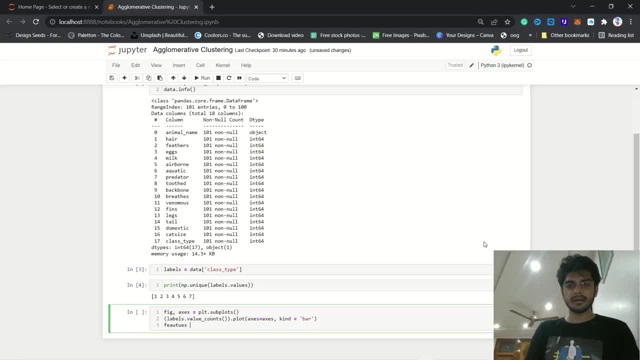 unsupervised learning. we go for features Like we categorize, We work with our data With some sort of features, Like different data have different kind of features. Let's say There are aquatic type animal which we want. That is a feature Like of animal. 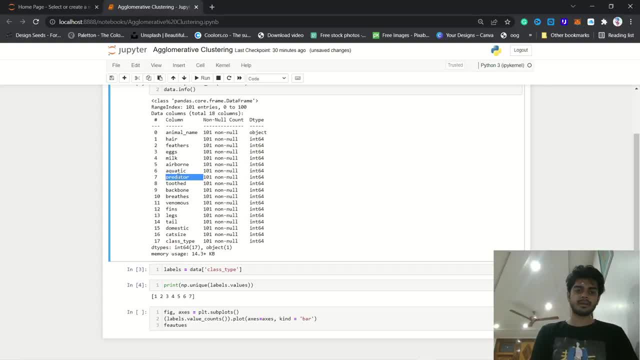 who are aquatic in type, Who are predator, Who are, Who have things, Who have legs. So we can use that, We can say features And that is a variable And I will say It will store dataValue. So what is the meaning of this? When we write a semicolon, It will. When we write this: 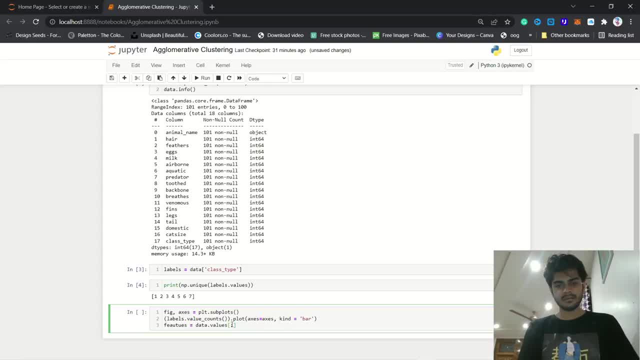 Let me explain this to you. So I am making a data frame And I will go ahead and let me write this Like old thing, Okay. So what does this mean? So this represent rows, So this represent row And this represent column, And I am saying that I want to store this. 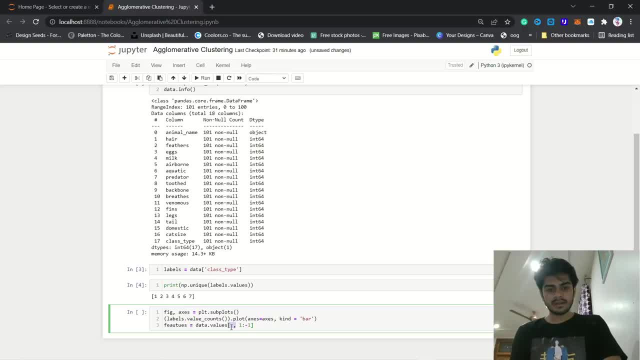 value in our feature. Now, what is this value? When we write a semicolon, It actually says that Take all the rows. Like, semicolon means take all the rows, All the rows as in: like this is row over, This is like horizontally, These are known as row. Vertically is column. 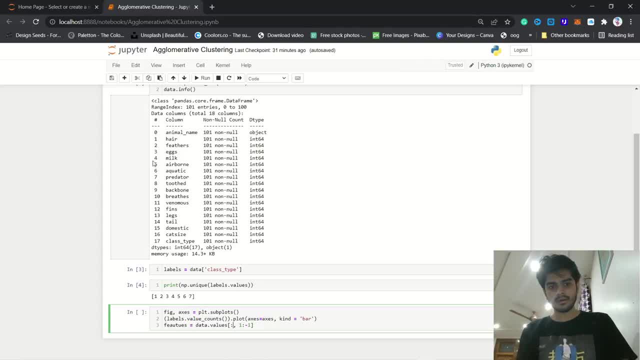 Okay. So I am saying that Take all these rows And we want column 1. And this is minus 1. Which is like last column from first. We want that. So we want all rows And we want first to last column Okay And store it into feature. 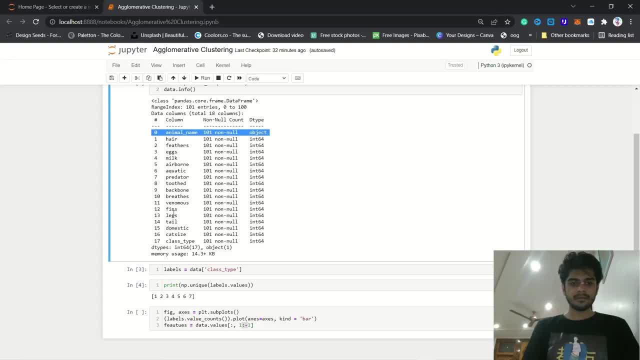 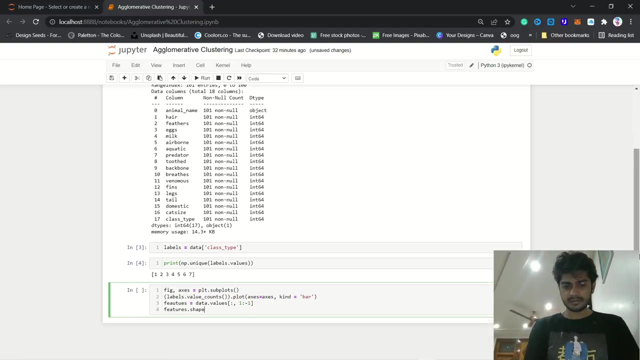 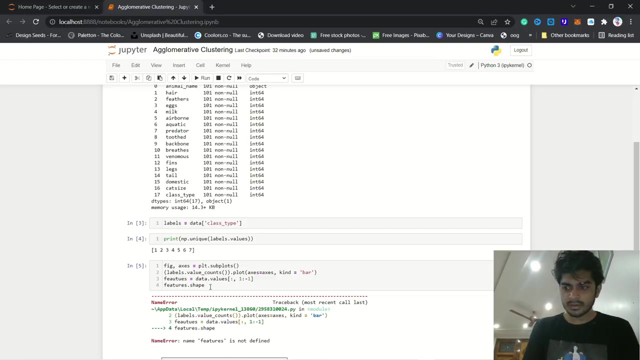 See, We want animal name And we want our cluster As a column. So we will take features And let's check shape of our features. Like, I think I should separate this code into two cells, But let's run that. So yeah, Features are known, different Feature. I think this. 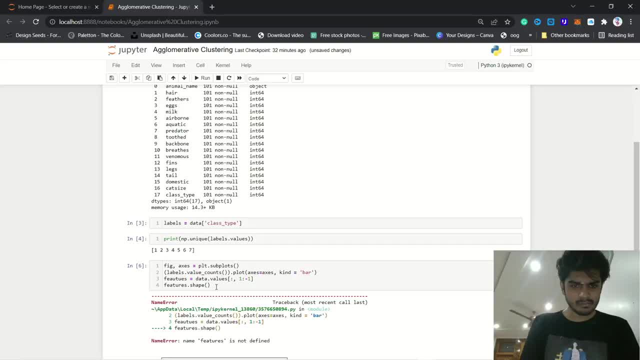 should work. Hmm, Okay, There is a spelling mistake. My bad, Because, as you can see, I like spelled this wrong And then that's why I am not getting it, Because I saw like F-E-A-T-U-R-A-S, F-E-A-T-U-R-A-S. 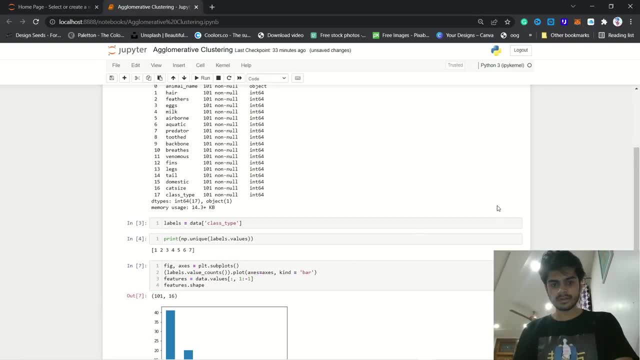 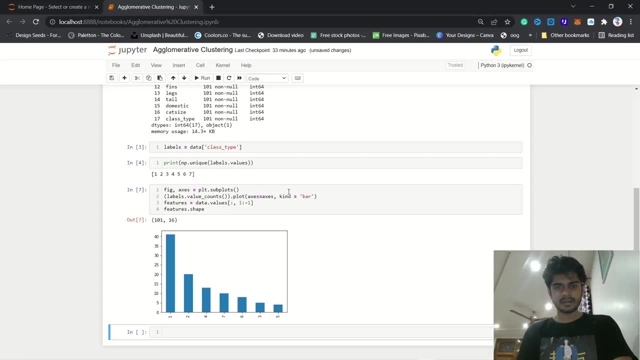 Now it should give us what we want. Yes, So we have our figure Which represents like axis And we like what is axis? again, Axis, we have defined somewhere, Let's say label dot value count. It is actually representing label data value count. What is label? Label is class type, Okay, And how many values are? 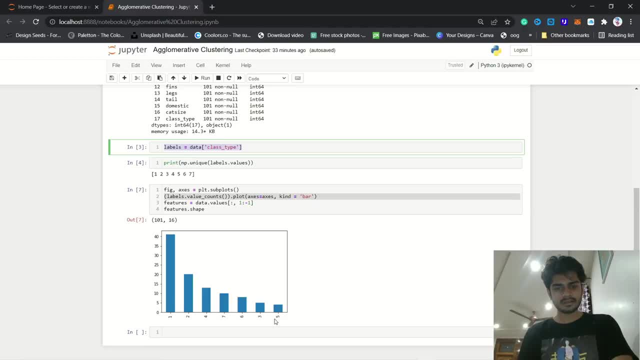 there Let's see 1,, 2,, 3,, 4,, 5,, 6,, 7.. And, as you can see that there are 1,, 2,, 3,, 4,, 5,, 6, 7 unique values. So there is this: 1,, 2,, 3,, 4,, 5,, 6,, 7.. And they have a value count. 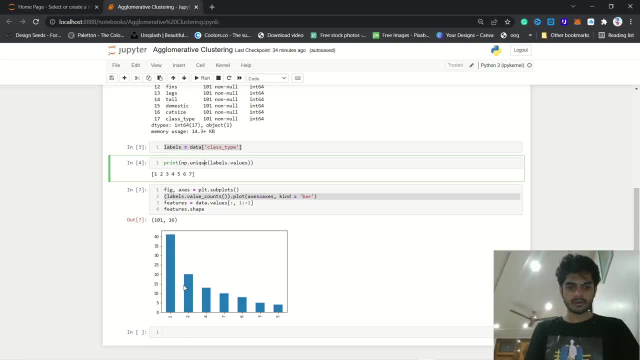 like: 1 have a value count of 40.. 2 have a value count of 20.. 4 have a value count of around 15.. 7 have around between 10 to 15.. 6 have around 10. I guess 5 is like 3 have. 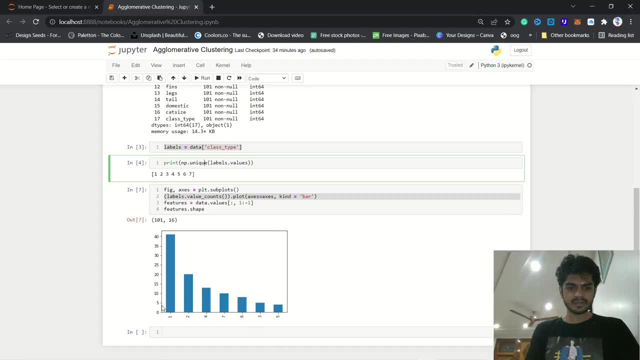 a value count of 15.. 6 have around 10, I guess. 5 is like. 3 have a value count of 15.. 6 have a value count of 5 and 5 has a value count between 0 to 5.. So this has given us the data. 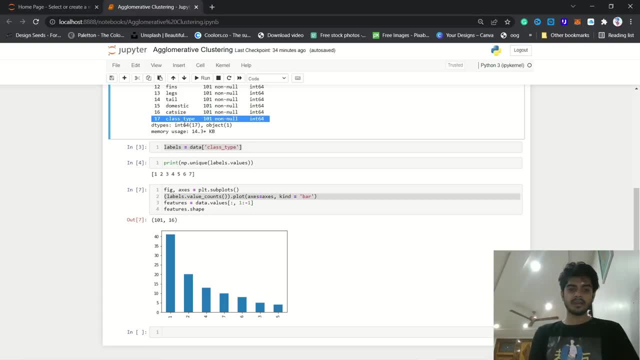 and the unique value which we have in our class type And the number of values which we have, And we have said that we want it into bar graph that we are seeing here. Then we said that features, number of features, how many features we have And we are taking. 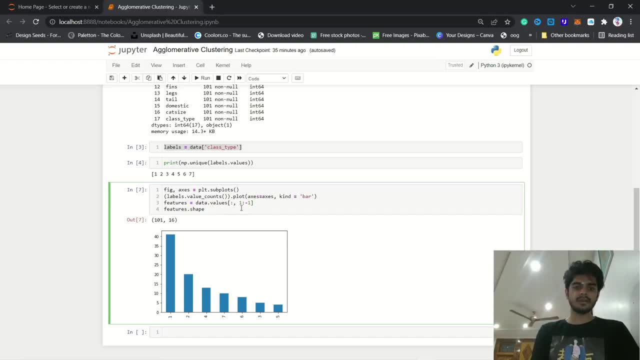 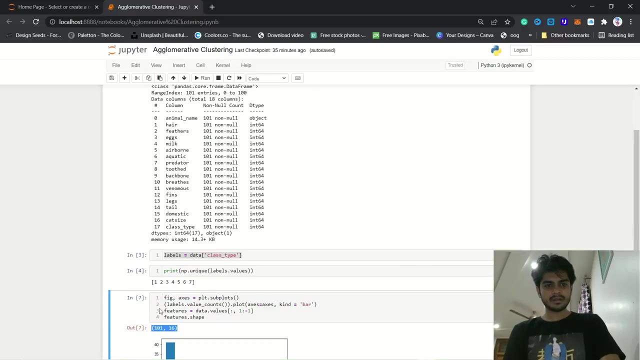 all the rows And this column 1 to minus 1.. And that is giving us this: Say, we have 101 rows and we are having 16 columns. How 16?? Like, we are like excluding minus 1 and we are starting. 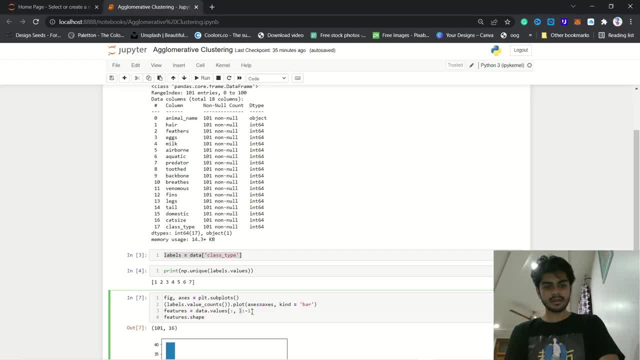 from minus 1 and we are going from like we are starting from 1 and we are going to minus 1.. So we are excluding this and we are excluding this. So these are the features we are taking. So, on total, we have 16 features, as you can. 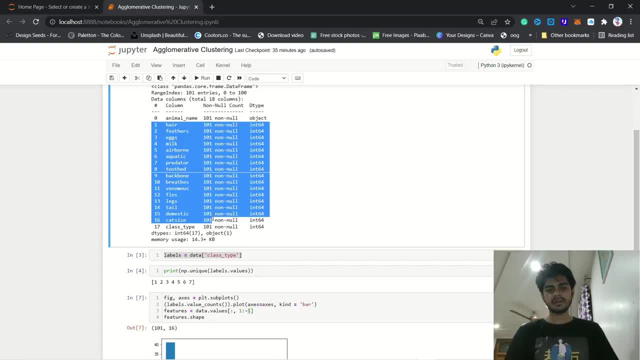 see. So we worked with our data. We saw what kind of data we have. We got the information of our data. We plotted unique values from our data. We got the shape of our features. How many features are there? How many unique values are there? In next video we will go.